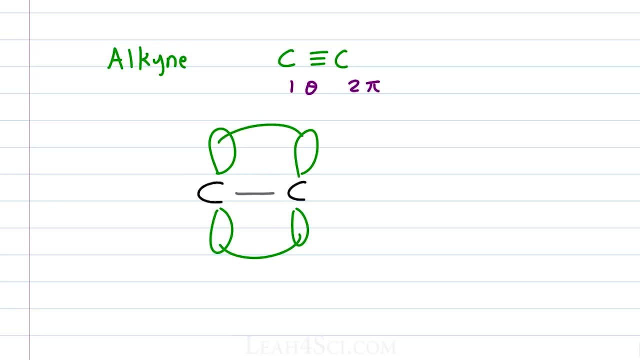 our first pi bond In the Z plane. we'll show another P orbital where the dark blue represents coming forward out of the page and the light blue represents going back into the page. When these overlap we get the pi bond in the Z plane. 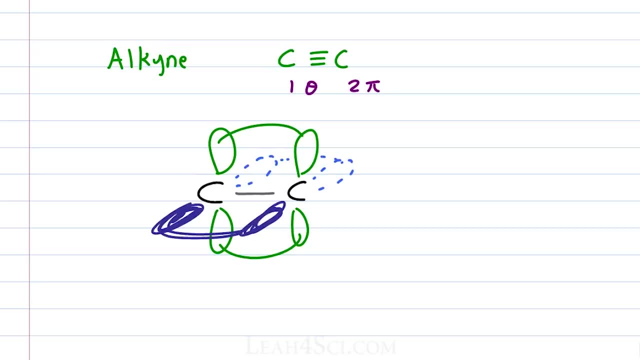 Carbon. having four orbitals, saving the Y and Z P orbitals for pi bonds, we're left with just one S and one P that fuse together, making the alkyne and SP hybrid, making the alkyne a linear molecule with a 180 degree bond angle due to the SP hybridization. 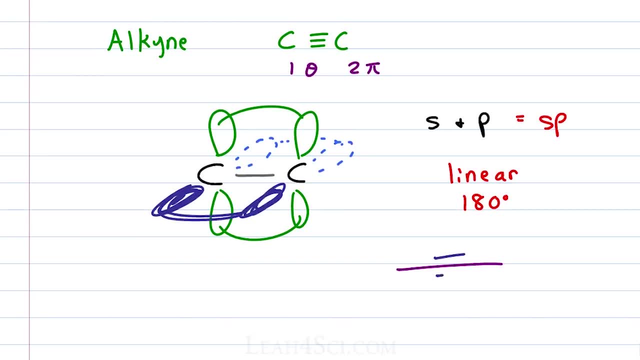 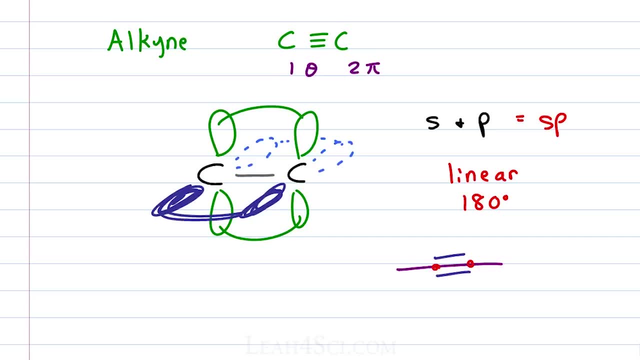 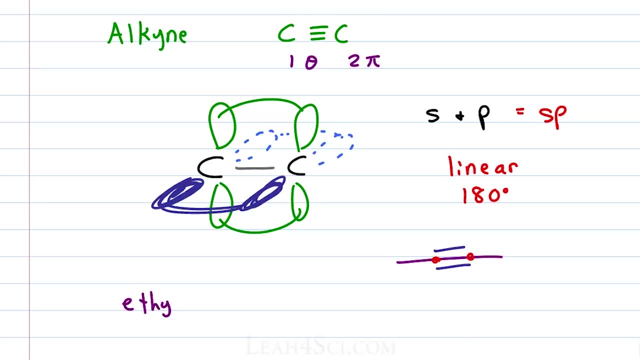 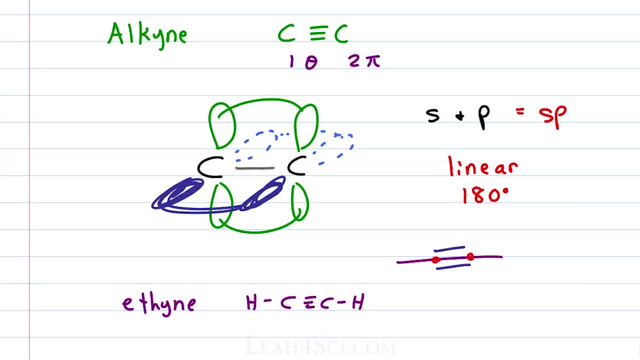 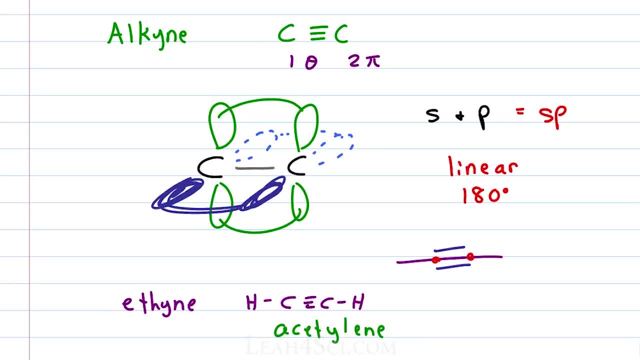 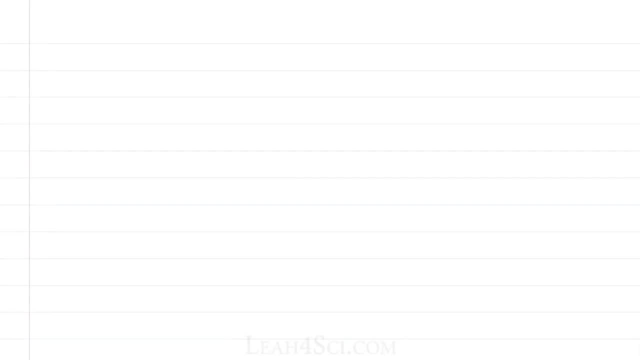 memorize this because it will show up over and over on your exams. For more in-depth review, make sure you watch the hybridization and naming videos link below. But what makes the alkyne so exciting for reactions? The first is the fact that alkynes are acidic. 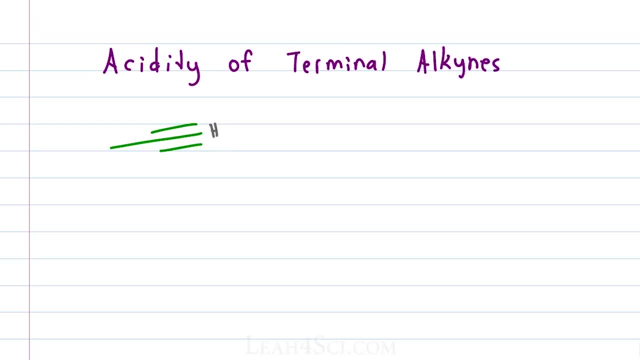 A terminal alkyne is when that has the alkyne at the very end of the molecule so that it ends with a hydrogen, rather than this end which has a carbon. This hydrogen here is fairly acidic, where acetylene, as we saw above, has a pKa of 25.. 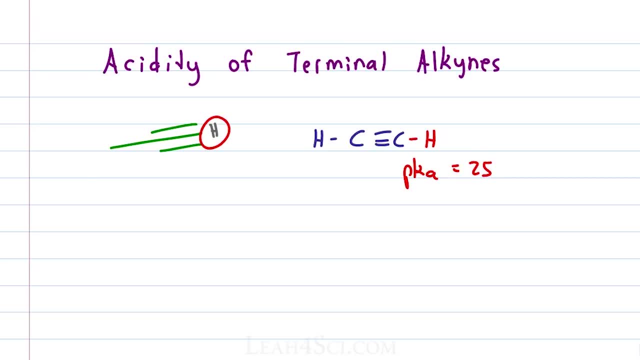 The pKa changes slightly depending on what else is on the molecule, but 25 is the general range. It's not too acidic, but it's definitely acidic enough to participate in reactions, For example, in the presence of a molecule. the pKa changes slightly depending on what. 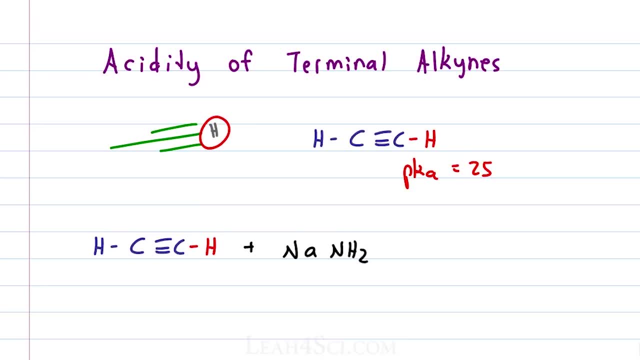 else is on the molecule, but 25 is the general range In the presence of a strong base like NaNH2, where Na plus is a positive spectator, leaving us with the amide ion. NH2 minus, the amide will reach out for and grab the terminal hydrogen. 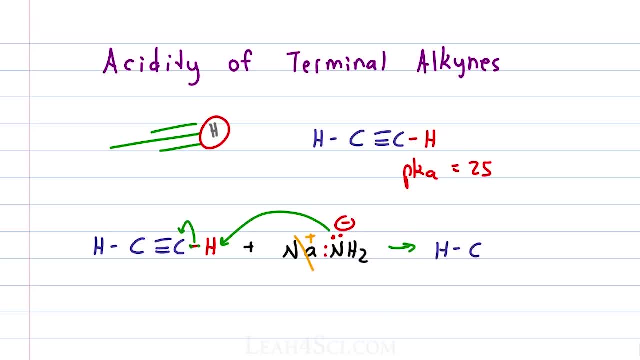 giving acetylene back its electrons and forming the acetylide anion along with NH3 in solution. The acetylide is a good nucleophile and a key to your retrosynthesis arsenal because you can now use this for SN2 reactions. You can now use this for SN2 reactions and chain elongation. 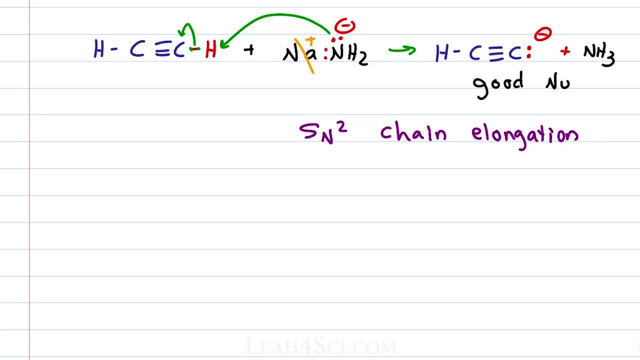 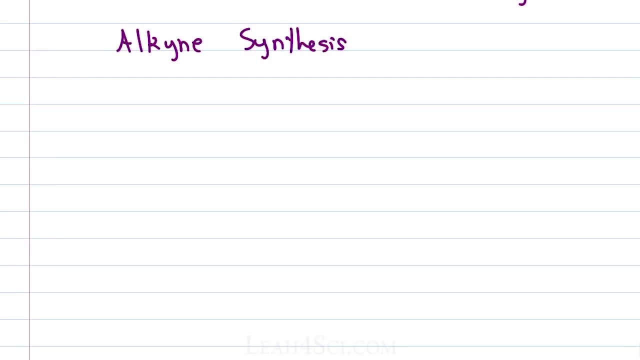 What else can we do with alkynes? Let's do a quick run through and then we'll go into the individual reactions in the upcoming videos. If you're not given an alkyne, no problem, just make it. You can make alkynes from a vicinal or a geminal dihalide. 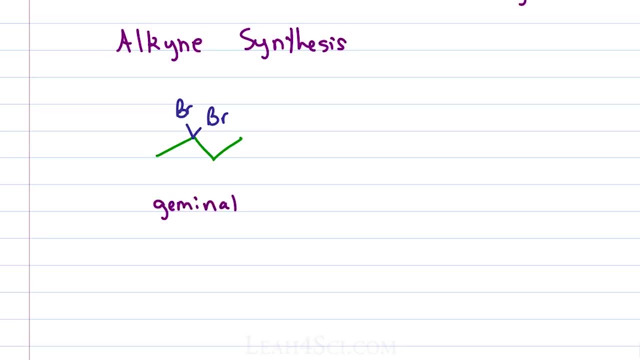 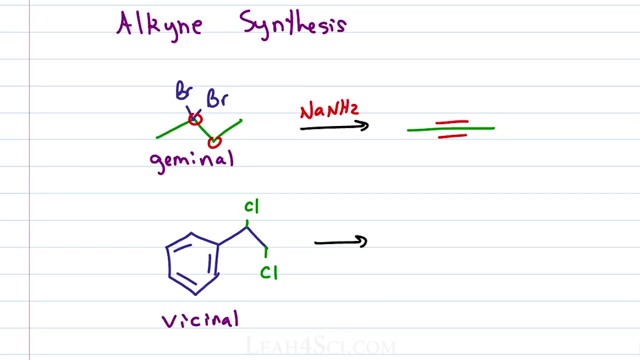 For example, here we have a geminal dibromide and in the presence of a strong base we get a double elimination. Okay, That gives us two pi bonds forming between these two carbons for an alkyne. We can also start with a vicinal dihalide. in this case we have chlorine on two neighboring 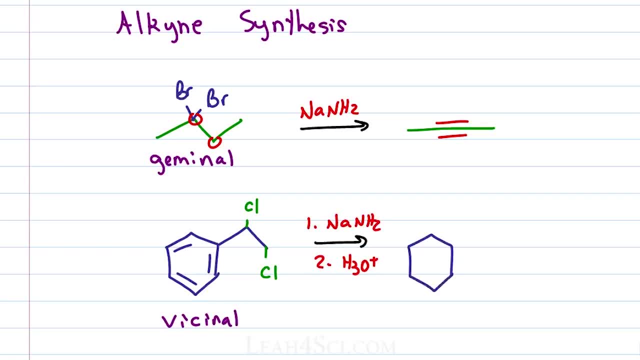 carbons and in the presence of a strong base, once again will give us an alkyne. In upcoming videos we'll look at why we need H3O plus when forming a terminal alkyne. Say we don't actually want the alkyne, but instead we wanna use it as a stepping stone. 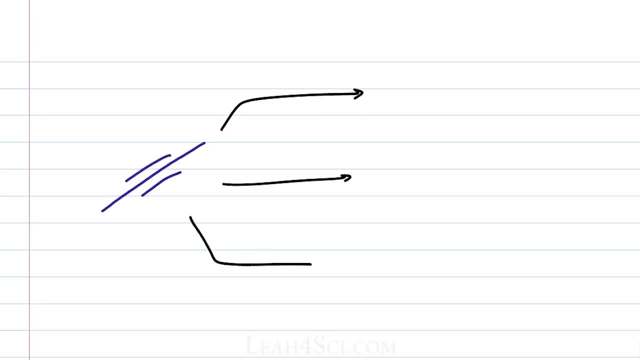 for other reactions, that's perfectly okay. We can reduce the alkyne if using H2 and a metal catalyst all the way down to the alkyne, or stop at the alkyne. Using H2 and a Lindlars catalyst, we'll get a cis-alkyne. 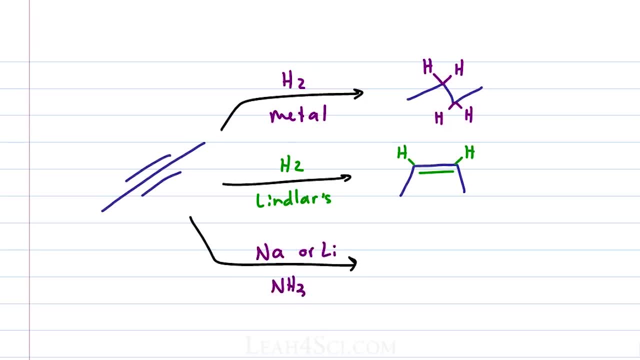 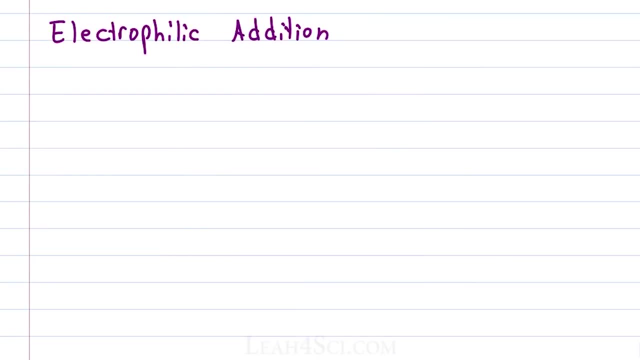 Using sodium or lithium in liquid ammonia for dissolving metal reduction, we'll get a trans-alkyne. And of course we can use the alkyne as a jumbo point for adding functional groups to the molecules. Okay, For example, we can react it with HX or X2 for hydrohalogenation or halogenation. 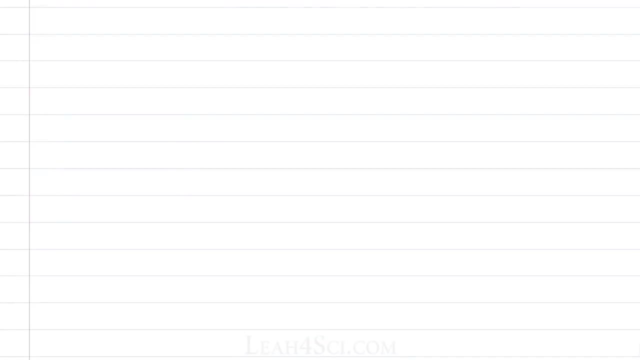 For example, using HCl or Br2.. We can do a hydration reaction which initially gives us an alcohol but then, through Ketoenol tautomerization, gives us a carbonyl. For example, if I use BH3 followed by H2O2 and NaOH.